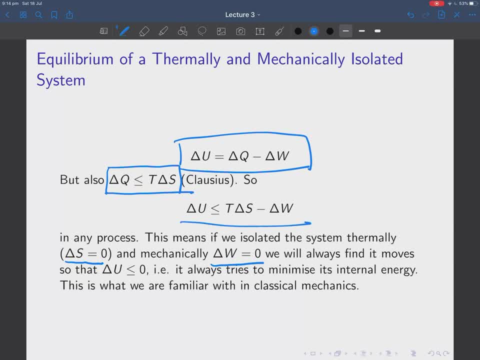 and when we do that, what we get is this the following inequality: That means du is less than or equal to Tds minus dw, which is that one. So we get an inequality. okay, What the hell does this mean? Well, this means that if we isolate the system thermally, 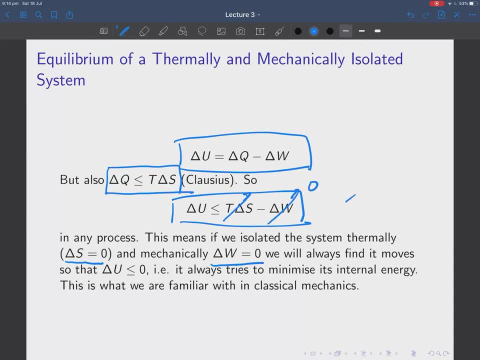 so that's zero. and mechanically, so that's zero. it will always move, such that du is less than or equal to zero. okay, In other words, it tries to minimize its internal energy. okay, So a system which is mechanically and thermally isolated. 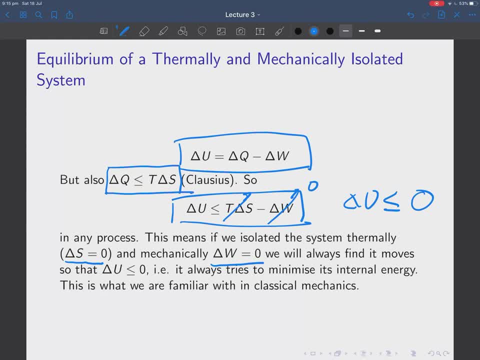 what it will do is it will try to minimize its energy, its internal energy. okay, And that's exactly what you're familiar with in classical mechanics. If I have a particle and a potential, here's my potential here: u versus x. 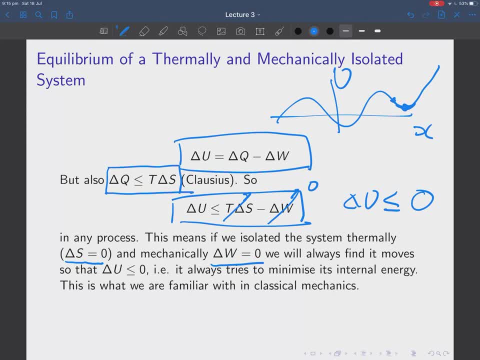 And I put the particle there and I apply a little bit of friction just for fun. it will go down here and sit at the bottom of the well, okay, It will always try and minimize its- locally, at least its- energy. okay. 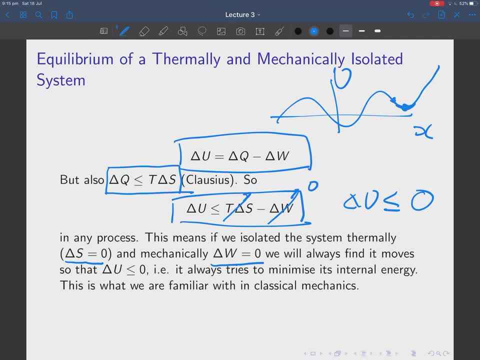 And you're absolutely familiar with this from classical mechanics. okay, You will note this particular law involves doing two things. It combines the first law and the second law Because the usefulness of the first law is completely obvious, I think, to most people. 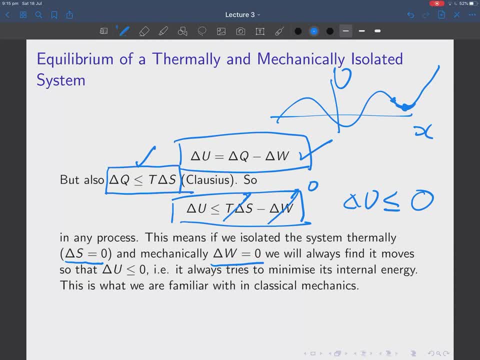 There's conservation, There's energy. But then you say: well, what about the second law? Where do we use that? Well, we're going to use it a lot here, And we're always using it in its inequality form, which basically says that the Q is less than or equal to TDS. 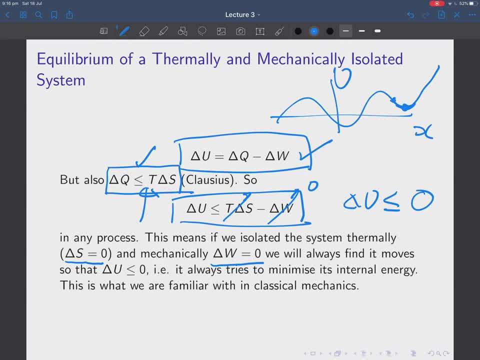 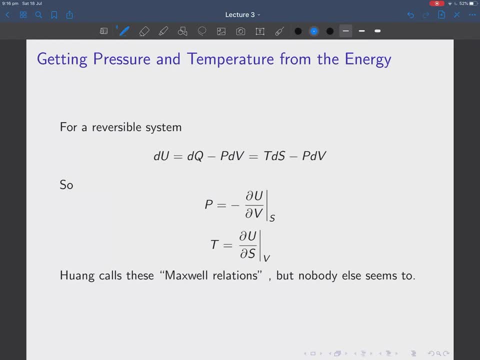 So when you put those two together, you find something which you know already from classical mechanics or from common experience in systems. You want a system that lacks its due equilibrium by minimizing its energy. okay, So that you already know, I hope. Now. 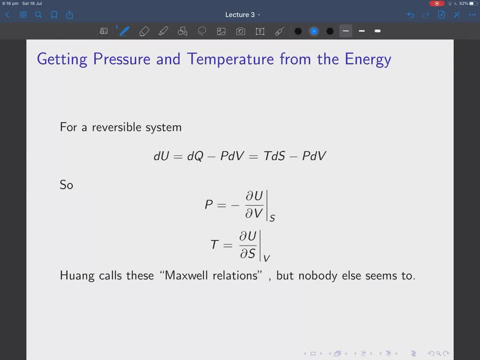 from our for a reversible system. we can get from this thermodynamic potential which we call the energy, the internal energy. we can get the pressure and temperature. So we know that DU is equal to DQ minus PDV. That's the first law. 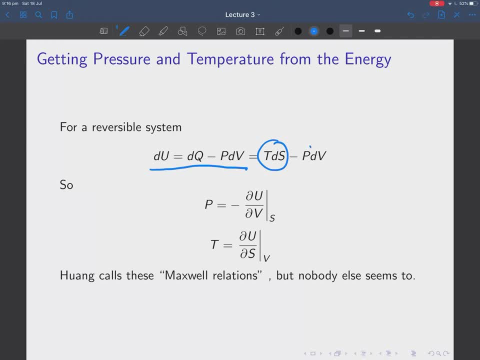 And DQ, if it's reversible, is TDS And PDV is pretty obvious, Okay, So from this we can just directly read off that the pressure here must be equal to minus DUDV at constant entropy And the temperature is equal to DQ. 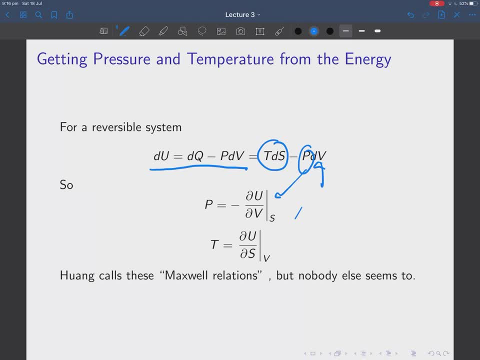 And DUDS at constant volume. Okay. So the natural variables here for U are S, the entropy and the volume. Okay, And if we do DUDV, we get minus P, And if we do DUDS, we get T. 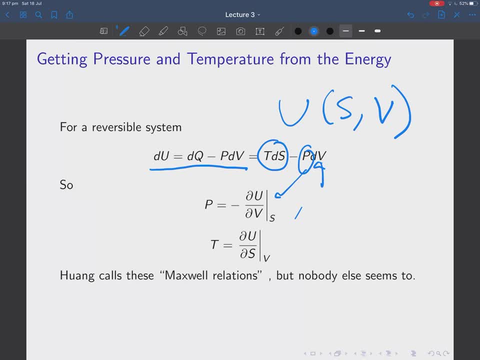 So you can automatically, from the equation for the energy, you can get off the pressure or the temperature of the system. Okay, One seems to call these the Maxwell relations. I wouldn't call them the Maxwell relations and I don't think anyone else would either. 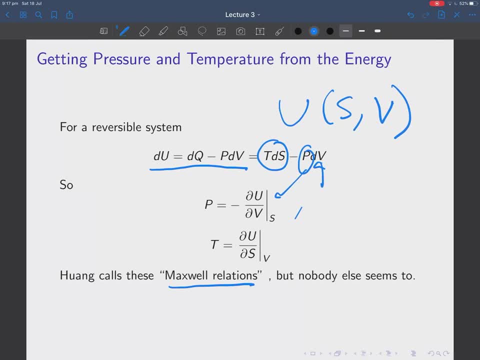 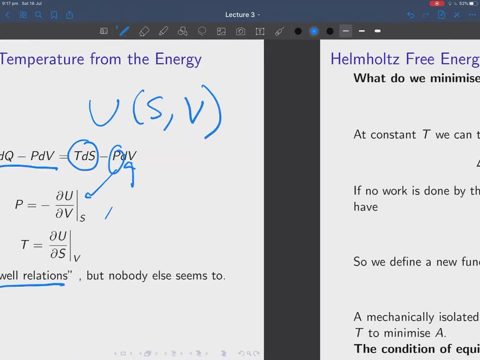 Maxwell, relations tend to involve second derivatives of things, not first derivatives, But you know we'll allow him to call them whatever he likes. But these are the relationships which give you the pressure and temperature in terms of the energy. Okay, Right. 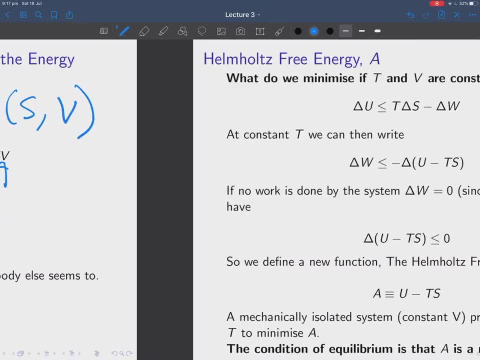 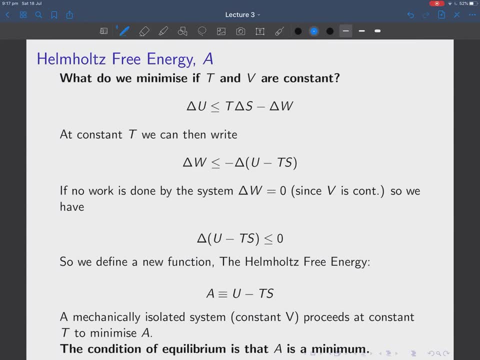 So this particular one, the energy, is what's minimized? if we have a system which is thermally isolated and mechanically isolated, Okay, That's good for some systems, but not all experiments, Okay, Okay, So if we conduct it in that way, what do we minimize if we have a system at constant temperature and constant volume? 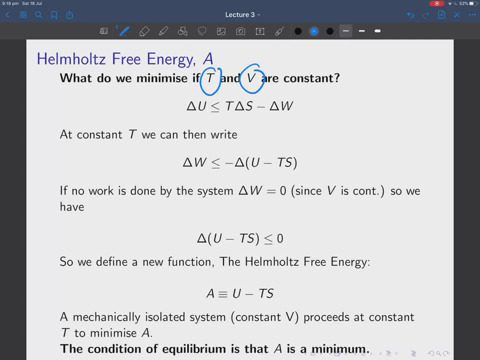 So I take my system and I say, oh right, I'm going to fix the volume and fix the temperature. What does it do? Okay, Well, okay, we can again write our inequality, which we had for the previous case. 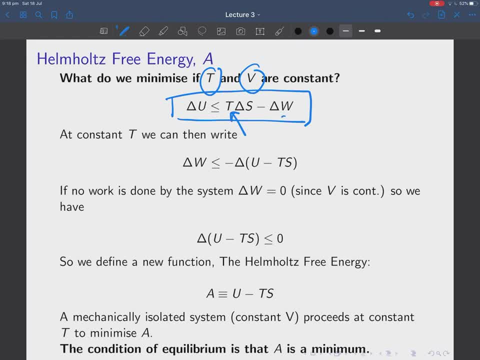 which is DU, is less than or equal to TDS minus DW, And if T is constant, which we can do, that, we can rearrange this and we'll get DW. And if T is less than or equal to TDS minus the change in U minus TS. 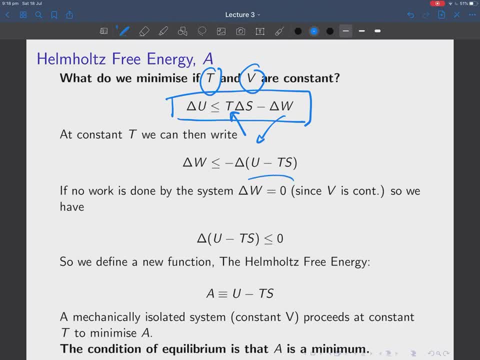 Okay, Now if no work is done, which we're going to say V is constant, so DW is zero. Okay, So DW is zero. We can then say: well, I can just write that as zero is less than or equal to minus delta, U minus TS. 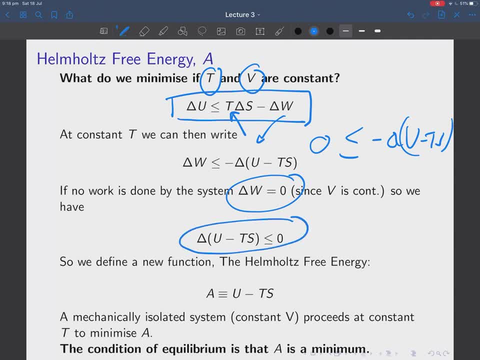 Okay, And then we'll flitch this around, multiply by minus one, We'll flitch the inequality sign around And we get this equation: Delta: U minus TS. So U minus TS is less than or equal to zero. And so let's define a new function, which we call the Helmholtz free energy, which is A. 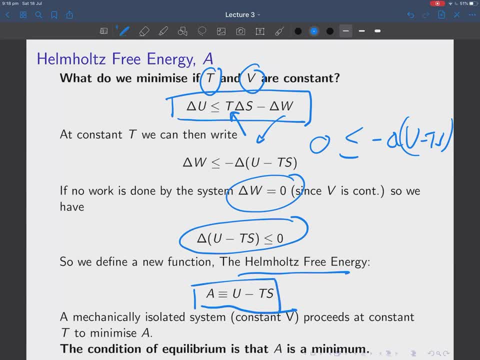 It's not written as F, but here it's written as A. A is U minus TS and a mechanically isolated system constant V and proceeds at constant T to minimize A. Okay, The Helmholtz free energy. The condition of equilibrium is that A is a minimum. 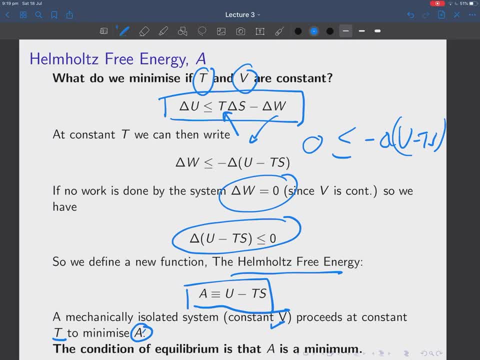 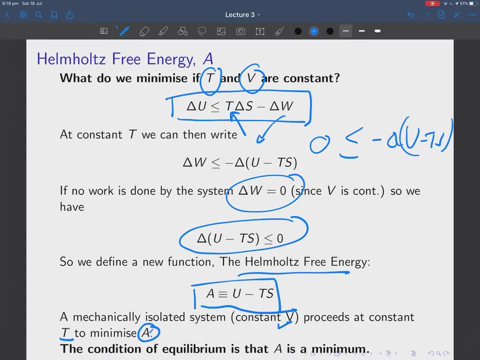 Okay, That's the condition of equilibrium. Okay, So if you have T and V constant, then you will minimize A. All right, So far, so good. Let's look at an example of this. You know what the hell does it mean? 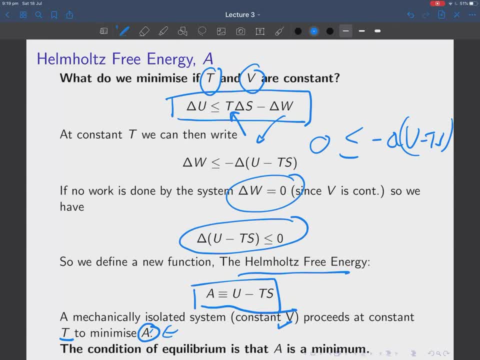 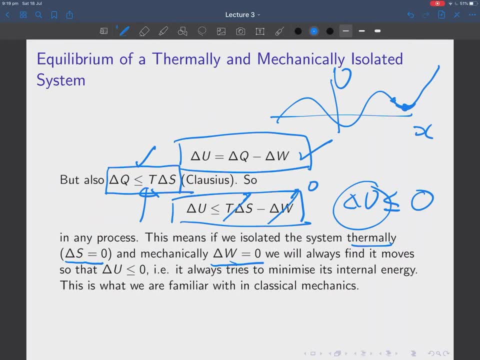 When you say this is minimized, it's minimized with respect to what. What's there to minimize? Okay? Well, what's there to minimize is it's minimized over all the free variables you have. So, for example, when we went back to the energy, if I have a particle in one dimension, 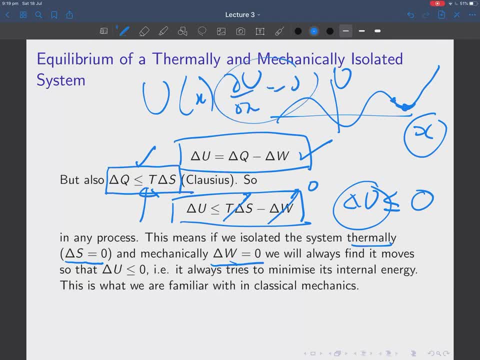 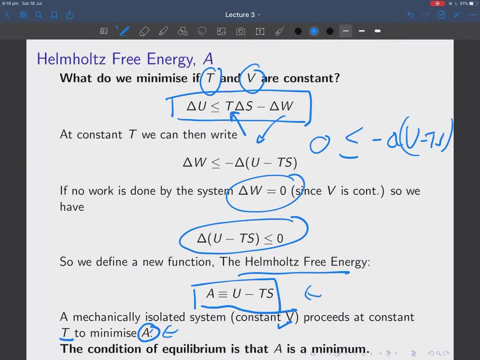 what does it mean to be minimized? Well, it minimizes over U of X, It minimizes with respect to X. So you have DU: DX equals zero, And so U is minimized with respect to our free variable, which is X. Okay, 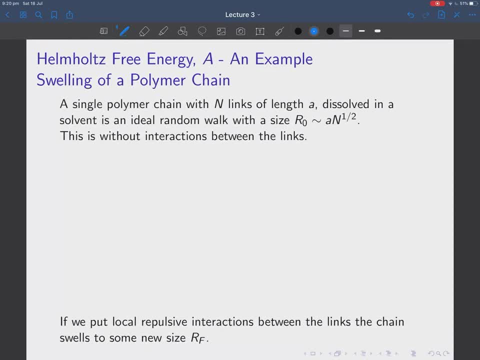 So, if we go to this system, what do we have to minimize over? Well, let's give an example. An example I'm going to pick is the swelling of a polymer chain. So a polymer chain is just a sequence of links like this: 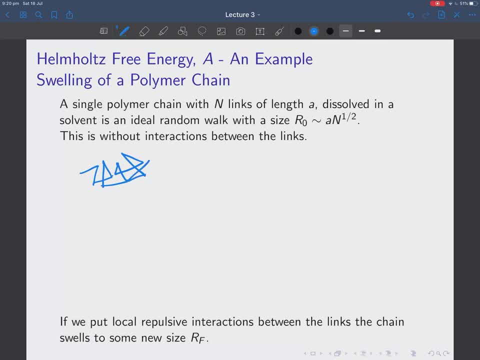 Here's the links. There are different models for polymers, but we're going to take the freely joined chain model, where it's just a whole series of links of length A and it does a random walk. Okay, And so if you have N links of size A and you dissolve it in a solvent 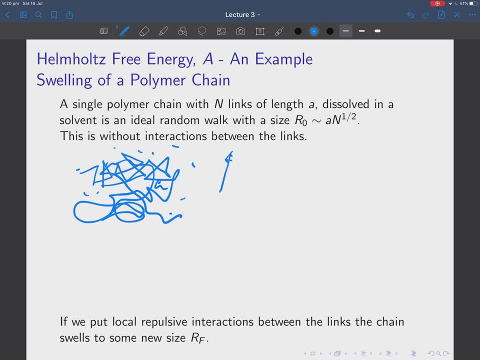 so the solvent here is one chain dissolved in a solvent and there are no interactions between the links. you find the size of your chain, which is roughly that size. there is given by roughly AN N to the half. It goes as the number of steps the half times the link length. 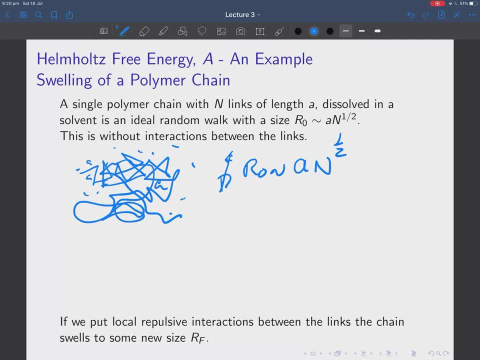 This is the link length: A, A, A And that's typical for random walk, as we've seen before and we will see many times again. Now that's the case where you have no possible interactions. Now, if we put in interactions between the links, the chain swells. 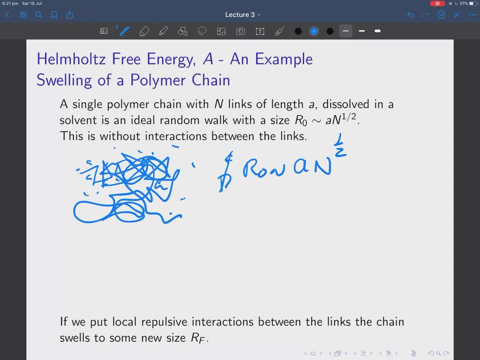 So what happens is we're going to put some local interactions. So between, say, this link here and this link here, there is some repulsive interaction. They're solid rods. They can't possibly occupy the same point in space. So if you have a polymer monomer and another polymer monomer, 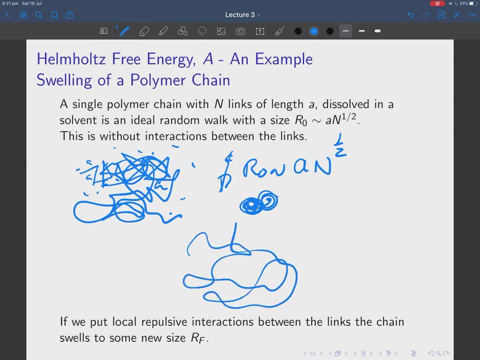 they will repel locally. okay, if it's in a good solvent And the thing will swell to some new size which is bigger. Instead of R0, we have some size radius RF. It'll be some size like that. We want to calculate how big RF is. 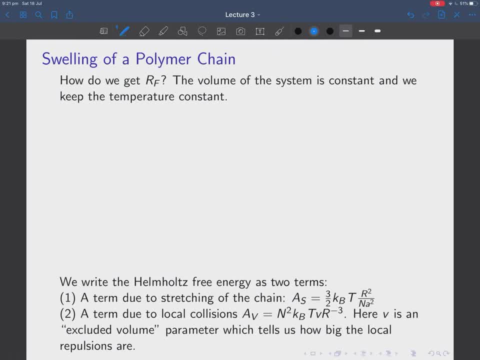 How do we do that? Well, what we're going to do is we're going to use the Helmholtz free energy for our chain. okay, The first thing you need to do is figure out what the Helmholtz free energy is. 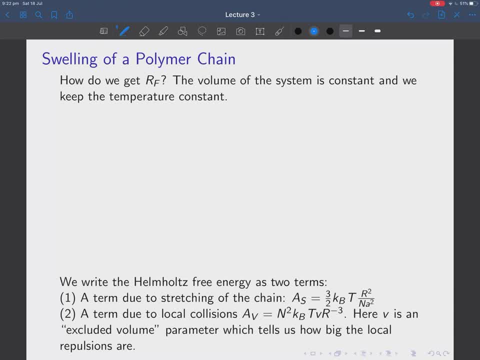 And you know that involves some statistical mechanics, okay, which goes beyond what we already know, okay, But we're going to keep the volume of the system constant and the temperature constant, okay, So the volume of our beaker? This isn't a beaker. 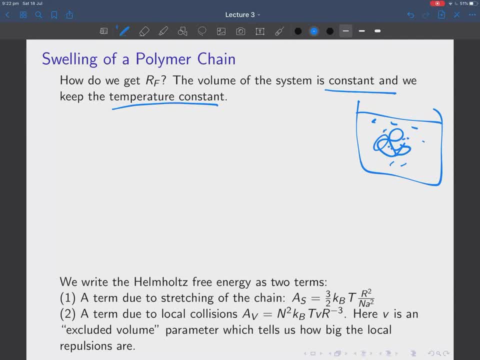 Here's a beaker. We've got one chain, just for simplicity. We've only got one chain with some solvent, And if it swells or de-swells it doesn't matter, because the solvent takes up some space as well, so the volume is constant. 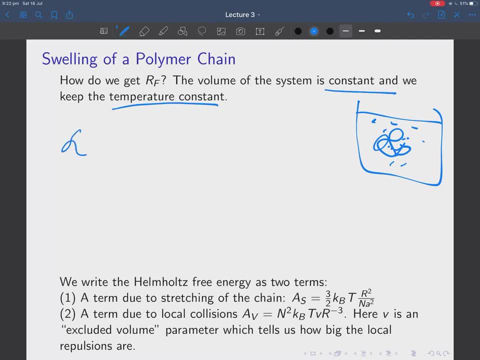 So we're going to write the Helmholtz free energy as two terms. The first term is due to the stretching of the chain. So the chain which is originally this big has now swollen to that big. okay, in terms of how big it is. 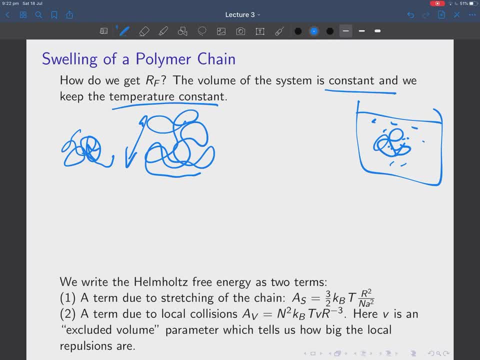 A number of monomers have stayed the same, but it's swollen a bit. okay, That involves somehow the chain expanding. It's expanding and stretching And when it swells to a particular size, r the free energy. you can calculate very easily. 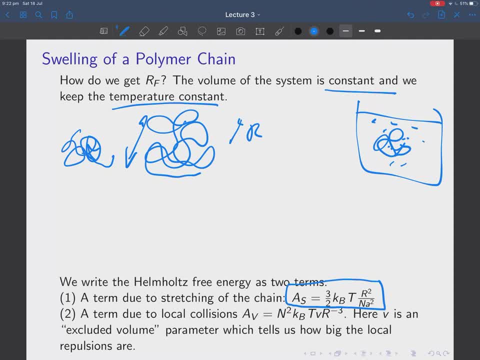 It's like a Hookean spring. It's 3kVt 3 on 2 kVt. the size squared divided by n, a squared just like half kx squared. basically, It's a Hookean spring. 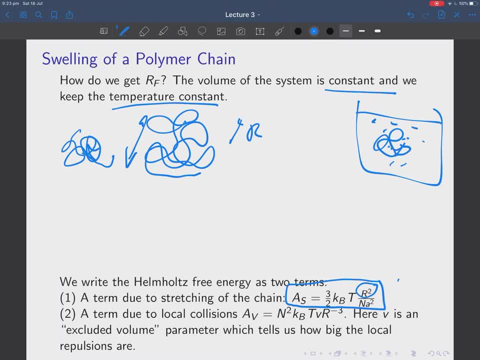 So if it swells to a size r, you get an extra part in the free energy, which is that, Of course, that particular term of the free energy if we're going to minimize it tells the system: look, don't swell. 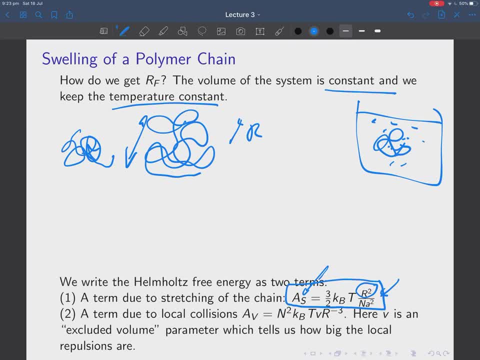 because as soon as you start swelling, r gets bigger and I pay a Helmholtz free energy penalty. Not good. There's another term, however, which makes it swell, and that term is the term which says: look this particular bit of chain here. 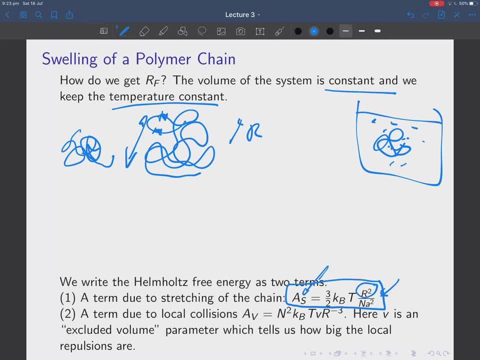 cannot occupy the same pushing in space as that part of the chain. okay, And that involves binary collisions. If we count all the binary collisions and we associate with each of them a sort of volume, what you find is that this particular term in the free energy is n squared. 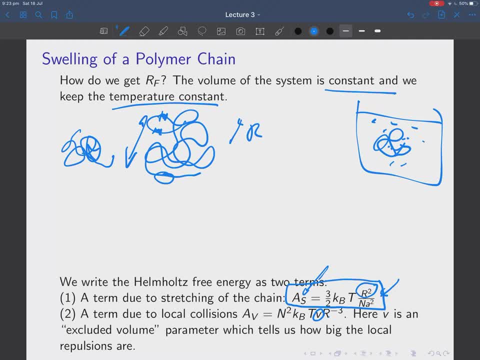 which counts the binary collisions: kvt. the volume element, the size of the volume element of this thing divided by the radius of my thing cubed, the radius of my chain cubed. okay, So we have two terms, that one and that one competing here. 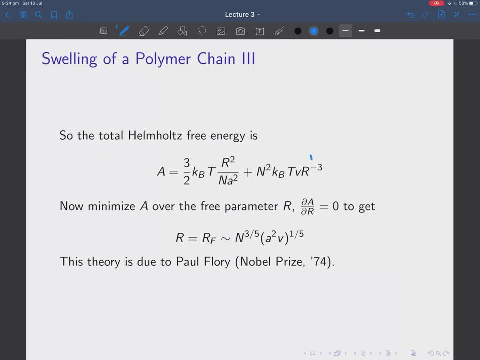 One of them says: make the thing smaller. one of the other says: make the thing bigger. okay, So the total Helmholtz free energy is the sum of those two, and to get the size of the chain, all we do is we take this. 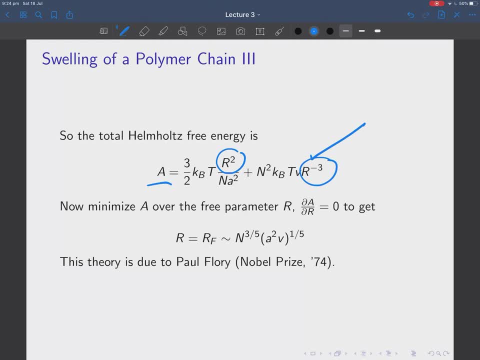 and we minimize over the only free parameter we have, which is r. So r can be anything we like, but we want to choose the minimum r. Helmholtz free energy says: choose the minimum r, just do dA. dr equals zero. 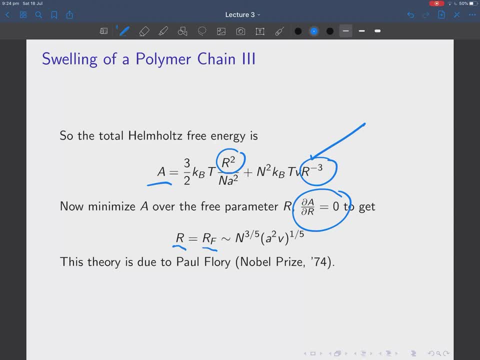 and we find, ignoring numerical pre-factors, that r, the minimum is at rf, which is n to the three-fifths, a squared v to the one-fifth, and in particular this n to the three-fifths law. 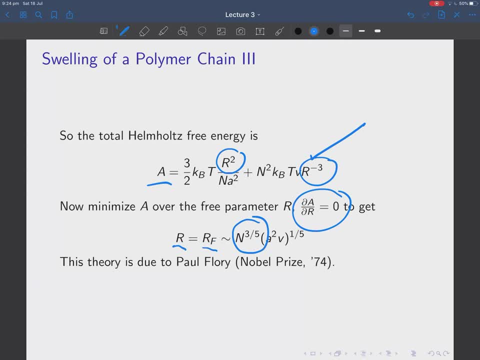 is what was seen here. You can experimentally, by many, many different measurements. you can do hydrodynamic measurements to measure the size of these things and do light scattering measurements, and when you put a chain in an environment which likes to swell up. 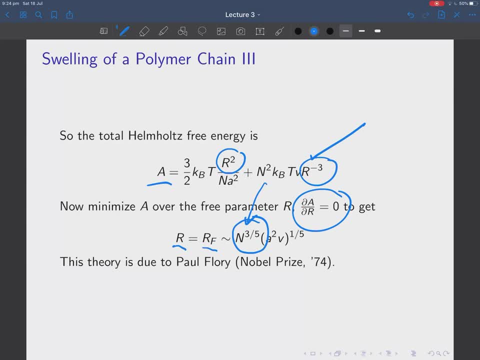 this is the size. It scales the number of monomers to the three-fifths, which is sizable because n could be for a chain. it could be 100,, it could be 1,000, it could be 10,000,, it could be a million. okay. 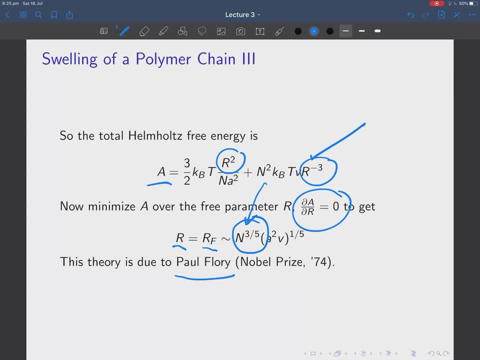 So it's a very, very sizable effect and this theory, which we just wrote down, is due to Paul Florey, who won the Nobel Prize in 1974, a long, long time ago, Okay, and Paul Florey was, in fact. 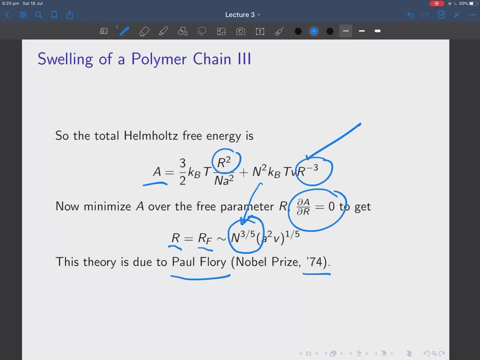 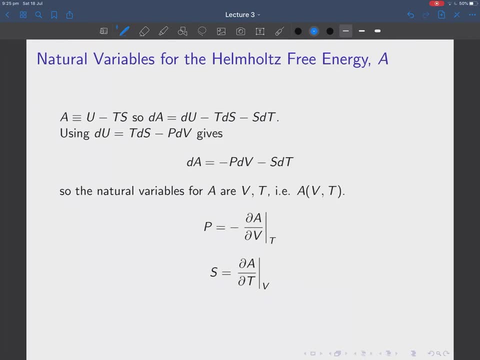 the postdoctoral supervisor of my PhD supervisor. okay, So Paul Florey is now unfortunately dead. Okay, so that's an example of using the Helmholtz free energy. Okay, what's the natural variables for this free energy? Well, the definition of Helmholtz free energy. 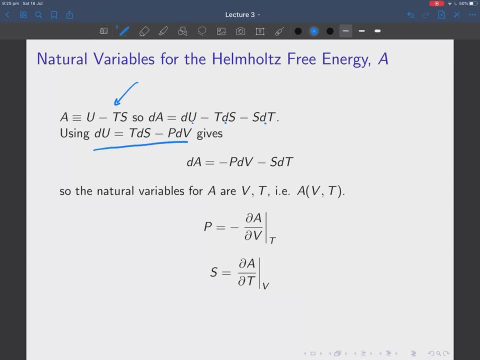 is U minus Ts and therefore dA is dU minus TdS, minus SdT, just differentiate this. But dU is TdS minus PdV, which is the first law, and so we get: dA is minus PdV, minus SdT. 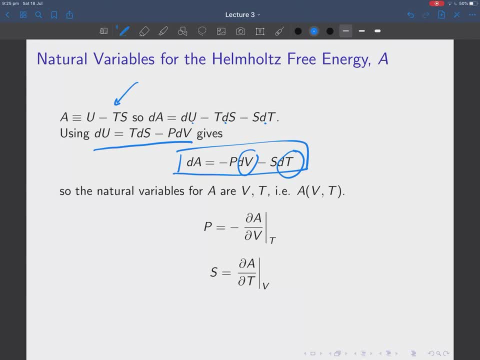 and so the natural variables for A are V and T. okay, And if you want to get the pressure, it's from here. it's pretty easy. P is minus dAdV and the entropy is dAdT. I think there should be a negative sign there. 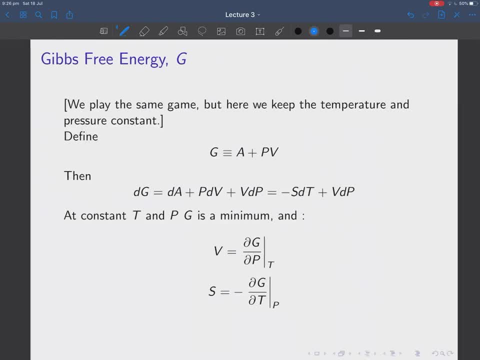 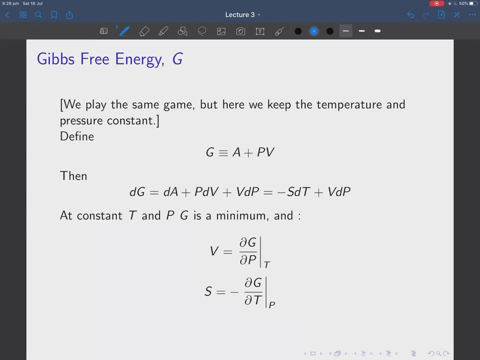 unless I made a mistake. Okay, probably a negative sign. All right, so that's the Helmholtz free energy. Next one: Okay, we're going to get the Gibbs free energy. So we're going to play the same game again. 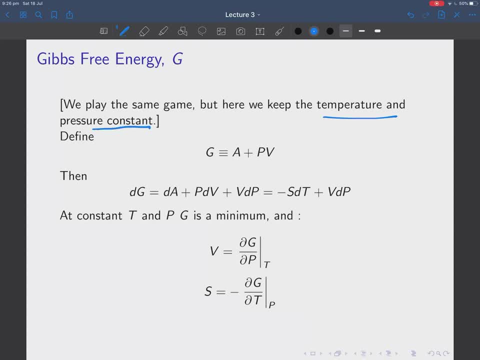 as we just did. but here we're going to keep the temperature and the pressure constant And if you do that and use the same algorithm we just did, you're going to use these inequalities. we can define the Gibbs free energy and that is equal to the Helmholtz free energy plus Pv. 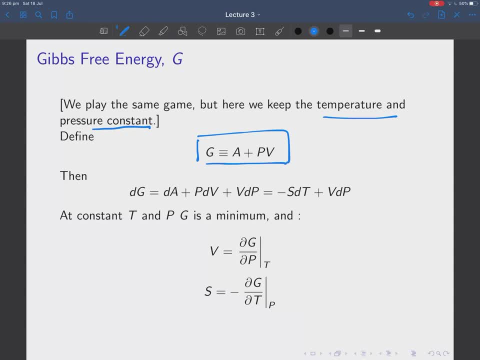 and that's what you minimize at constant temperature and constant pressure. Okay, I'm not going to derive that for you, but you can see. if you go back and do the calculation, that's what you'll get. And if we do dG. 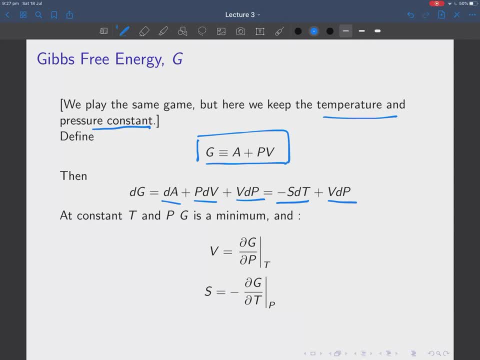 we find it's dA plus PdV plus VdP, which turns out to be minus SdT plus VdP, and therefore at constant T and P. G is the minimum. Okay, so that's what it is. 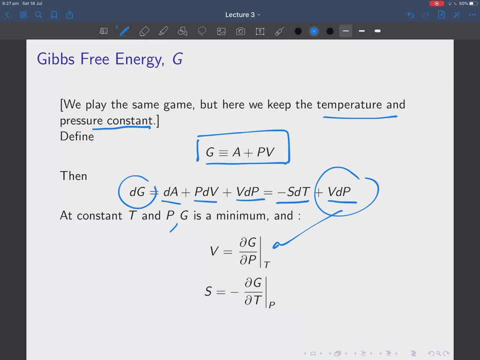 And then from this you can just read off directly: V must be equal to gdP and S must be equal to minus dG dt. Okay, constant pressure. Okay, that's the Gibbs free energy. Now, there's not much point in doing the Gibbs free energy. 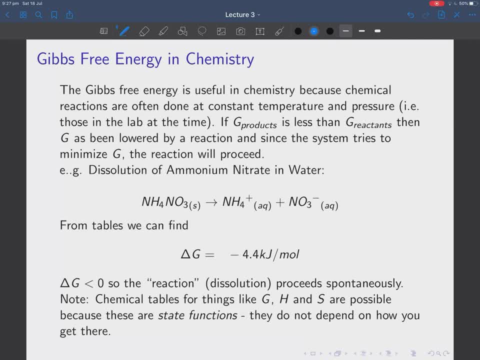 unless we actually do an example. Okay, and the example? that's really important. it has many applications in physics, of course, but its real usefulness is in chemistry, Because chemical reactions are often done at constant temperature and pressure, ie the temperature and pressure of the lab. 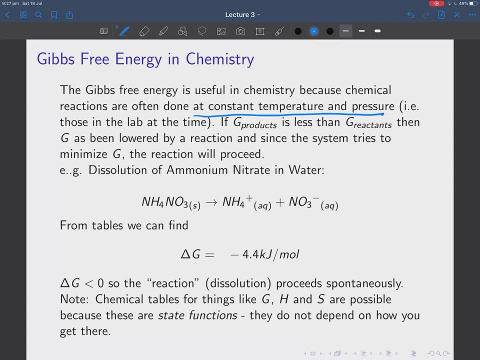 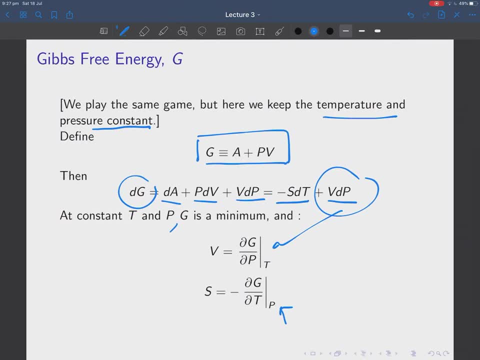 Okay, so that's why this is so useful in chemistry, because you have the lab's at 25 degrees, there's an atmospheric pressure, so we, you know, we're just going to use the Gibbs free energy to figure out what's going on. 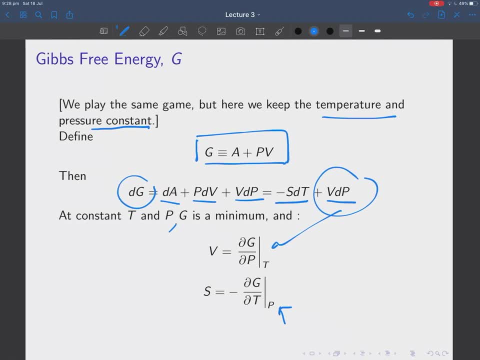 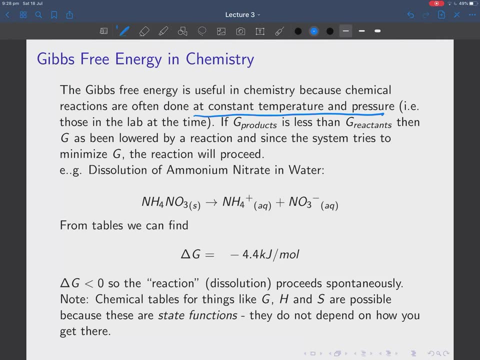 Now the Gibbs free energy thing tells us the chemical potential given by the Gibbs free energy. tells us that G is that systems try to minimize systems try to minimize G. Okay, try to minimize it. Okay, what does that mean? 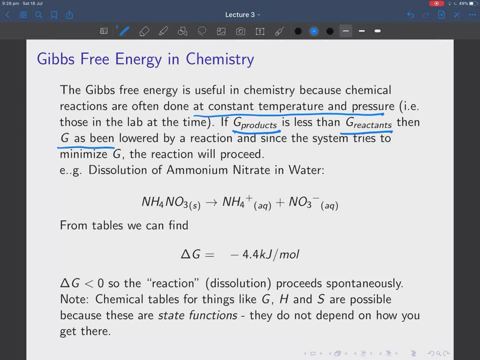 Well, that means if your G for the products is less than your G for the reactants, then G has been lowered by the reaction. Okay, and since the system tries to minimize G, the reaction will proceed. So if you have the products of a reaction, 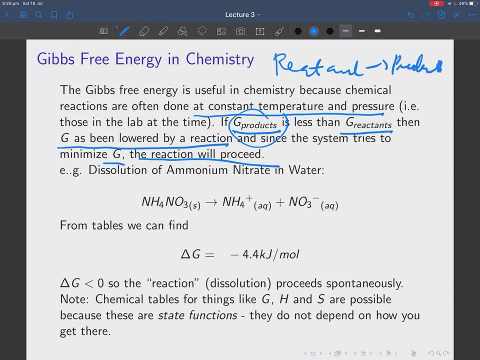 so you have here. we have reactants- goes to products. If this side has lower Gibbs free energy than that side, then the system will say: thank you very much. this is exactly what nature wants me to do: lower G, I will proceed. 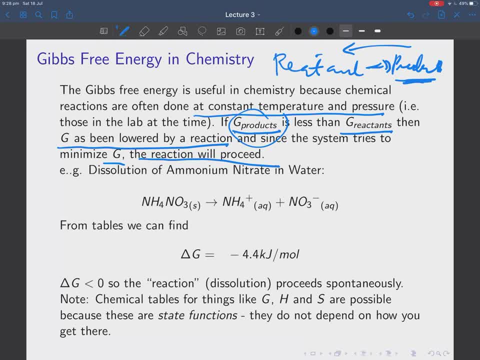 I will make this reaction go Okay. on the other hand, if it's the other way around, then the reaction will go backwards. Okay, so let's do an example here, A really simple example, which is almost not even chemistry. 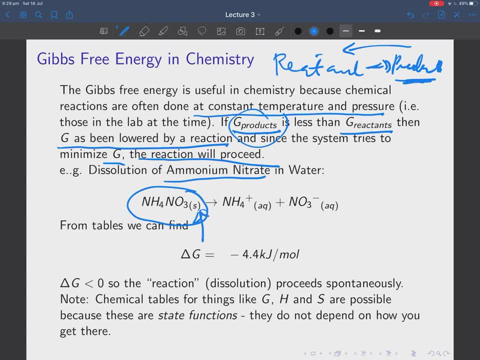 It's dis-dissolving ammonium nitrate in water. So ammonium nitrate is this stuff: NH4NO3.. It's a solid, solid stuff. It's used as a fertilizer, of course, And if you do, mix it with various other things. 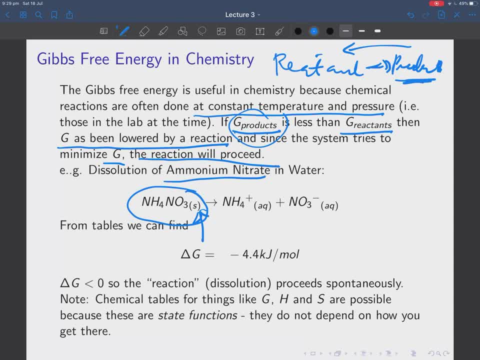 you can make an explosive out of it, Okay, And of course you know that's done. you know, in warfare, often ammonium nitrate is used as an explosive or used to be Okay. so what happens? we're going to take this stuff. 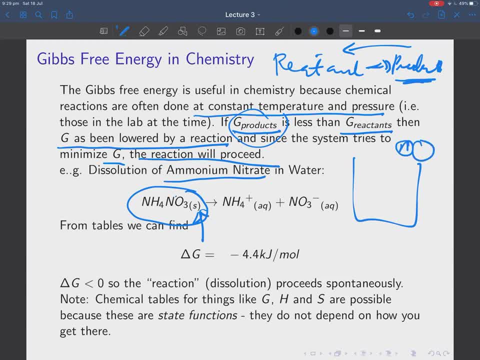 and dissolve it in water. So when it dissolves in water, here we go. I take some of this stuff. here's my ammonium nitrate. this is ammonium here and the nitrate bit And what it is. it breaks up into ammonium ions. 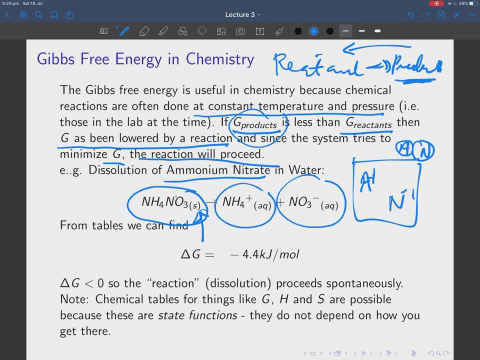 and nitrate ions. Okay, And there they are, floating around in water. So it's aqueous environment. So this is almost not a, as I say, not a chemical reaction. but you know, it depends on how far you're prepared. 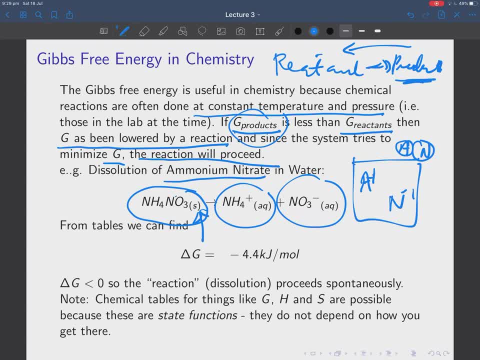 if you push chemistry. Anyway, you take this stuff, throw it in water. what happens? Well, you can go and look up what the delta G is for this reaction in tables. And it turns out to be. even if you can't look it up, 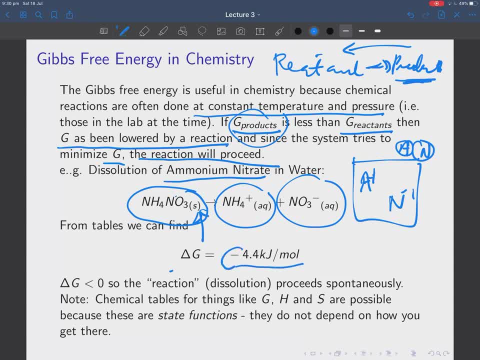 you can certainly calculate it from the tables, minus 4.4 kilojoules per mole. Okay, That tells us this negative sign here tells us something really important. The reaction, which is dissolution, proceeds spontaneously. It will just go. 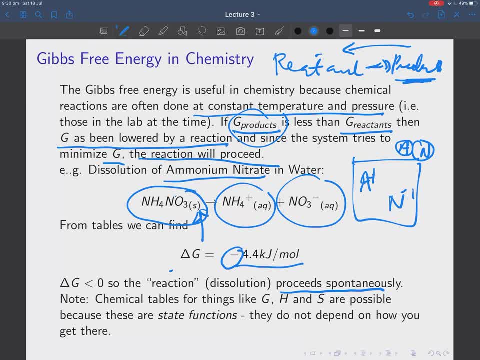 Okay, And so that tells us this reaction will happen: If you put ammonium nitrate in water, it will dissolve, Okay, It won't. just it doesn't spontaneously undissolve out of water and precipitate, Okay, So 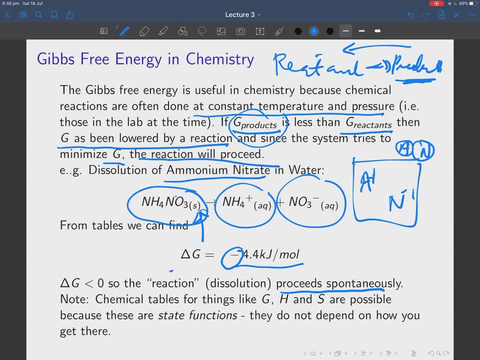 as an aside, you'll know there are these chemical tables in chemistry- Most of you must have done a lot of chemistry- And there are chemical tables which will give you G and they'll give you H, and they'll give you S or allow you to calculate. 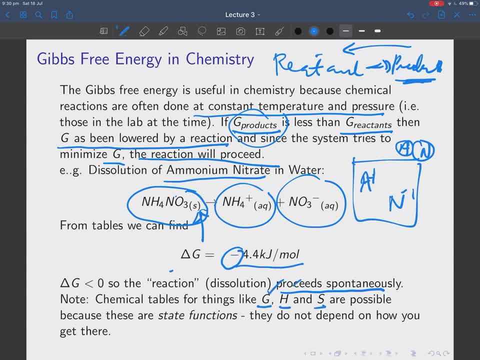 all those things for different reactions, And the reason why those tables are possible is because those three things are state functions. They don't depend on how you get there, Okay, So it's really important that you know. G H. 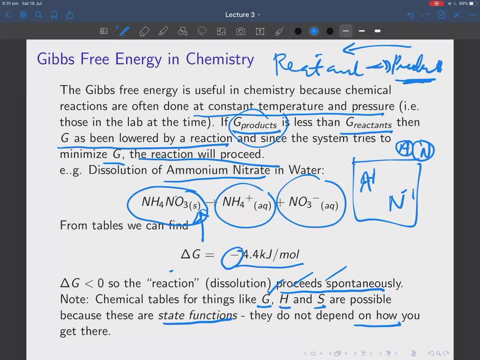 and N are seen are state functions. Otherwise you couldn't have these tables. Otherwise, for instance, the idea of Gibbs free energy would be very, very useless in chemistry. Okay, G, H and S are basically like the mass of. 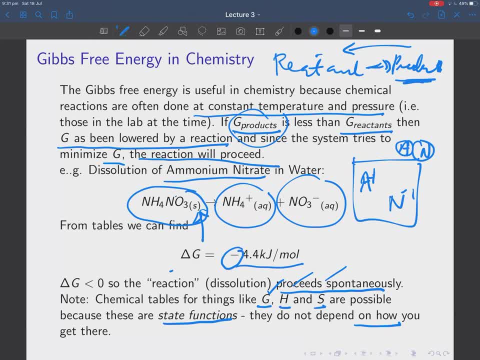 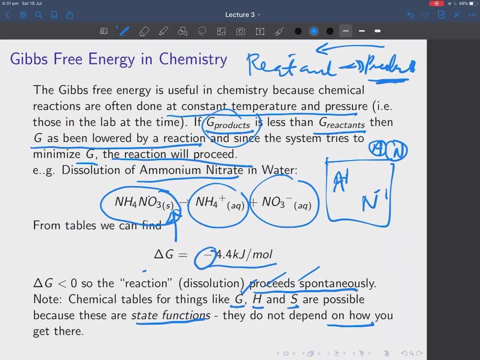 you know they're like the mass of oxygen. Okay, The mass of oxygen atom doesn't depend on how it got there. Okay, It's. you know, it's just the mass of an oxygen atom. So this is true in chemistry. 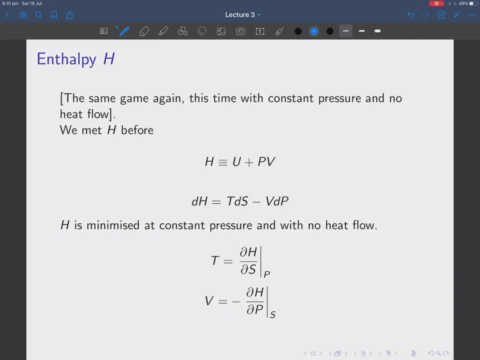 Okay, If delta G is negative, it proceeds. Okay, Now we can play the same game again and derive the entropy- Sorry, not the entropy, the enthalpy- And this time we're going to keep the pressure constant and have 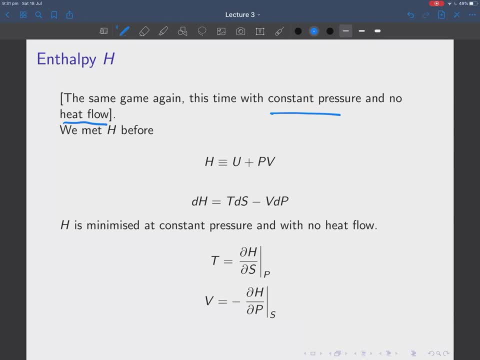 no heat flow. Okay, That's not usually the case in chemical reactions, but we'll see that the entropy still is important in chemistry. Okay, So we've got T plus PV. So it turns out that dH is T? dS. 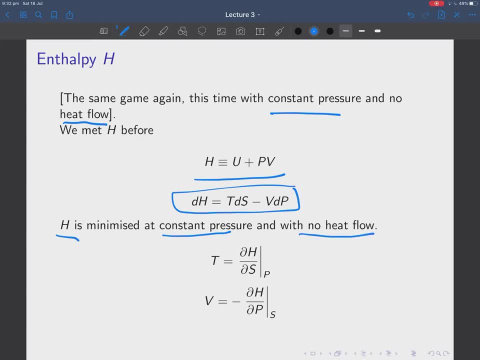 minus V dP, if you do the calculation based on the first law, And H is the thing that's minimized at constant pressure with no heat flow, And from here you can derive. you know, dH dS must be T and dH dP. 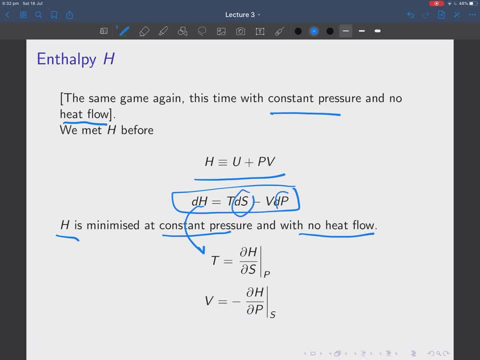 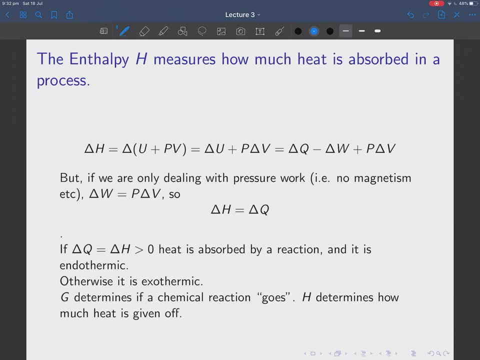 must be minus V. Okay, So you can get from those the temperature and the volume. All right, Natural variables here for H, Okay. So why is H useful? Okay, The entropy, Okay. It's useful because it measures. 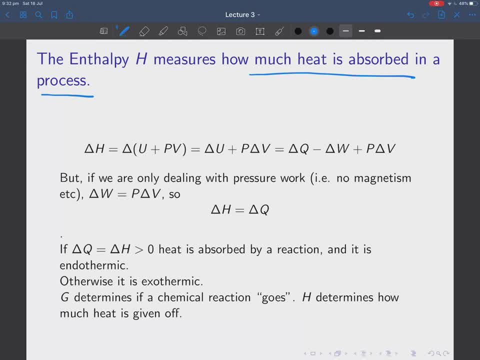 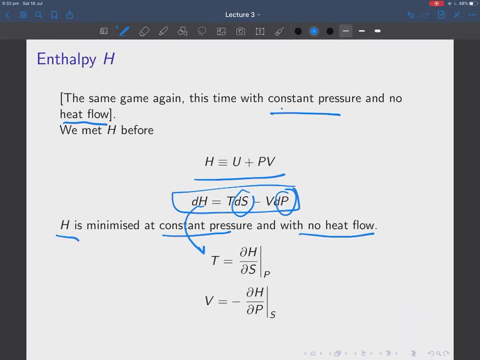 how much heat is absorbed in a process, in a chemical reaction for example, or even a physical process. So dH, by definition, is dU plus PV, And that's equal to delta U plus P, delta V. And why don't we have 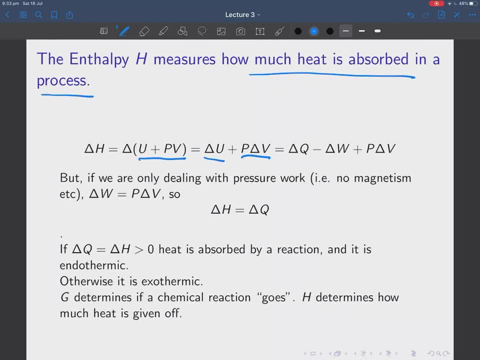 a, V delta P. Well, we don't have a P because we're going to have constant pressure for this system. Okay, As you get in the lab. Okay, Which is dQ minus dW plus P delta V. But if we're only dealing 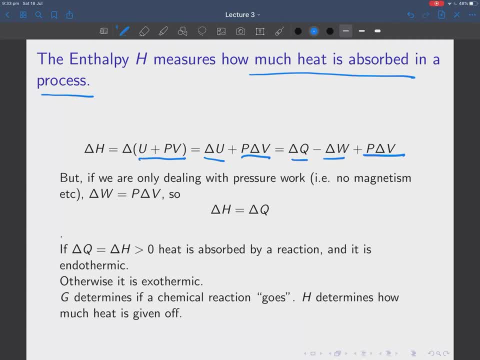 with pressure work. ie there's no, you know, no magnetism or any other kind of weird work, no electrostatic work going on, nothing else that's weird. then we have dW is PdV And those two terms. 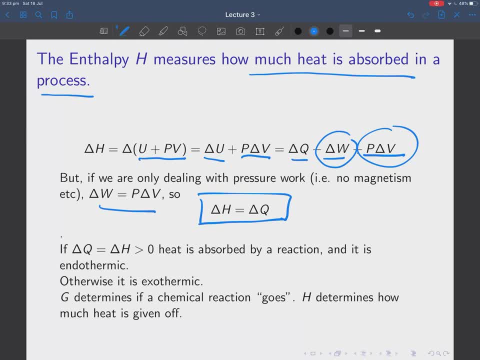 will cancel out, And so we have dH equals dQ, So dH. delta H is a measure of how much heat is absorbed in a reaction by the reaction itself. Okay, So now it becomes slightly tricky. It's slightly. 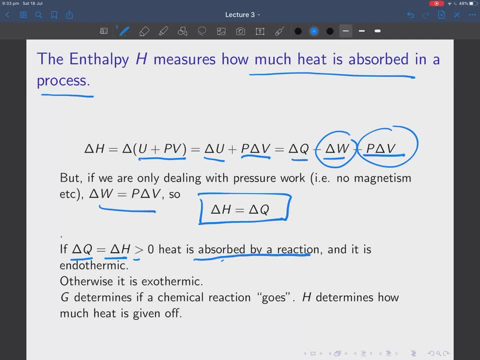 only slightly tricky, but you've got to think about what this means. If delta H, which is the same as delta Q, is positive, heat is absorbed by a reaction and it's endothermic. Okay, If delta H is bigger than zero. 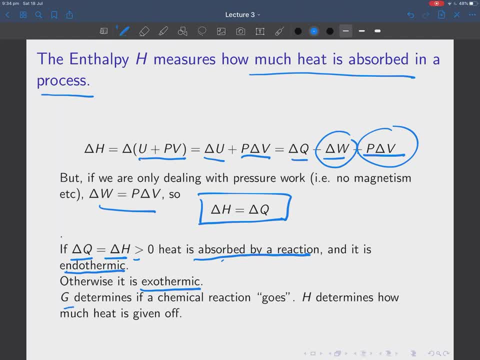 means reaction is endothermic. Otherwise, if delta H is less than zero, it's exothermic. Okay, So, as a summary, G determines if a chemical reaction goes forward and H determines how much heat is given off. Okay, 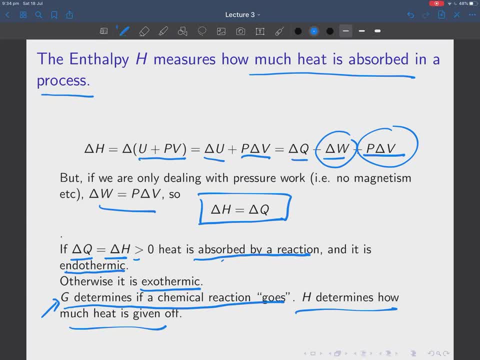 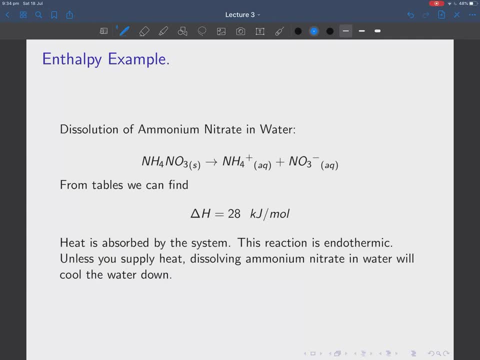 G is the important one in some sense, because G really says: is this a viable reaction? Okay, To some, to some degree, Whereas H tells you basically how much heat it requires. So let's do an example, We'll go back. 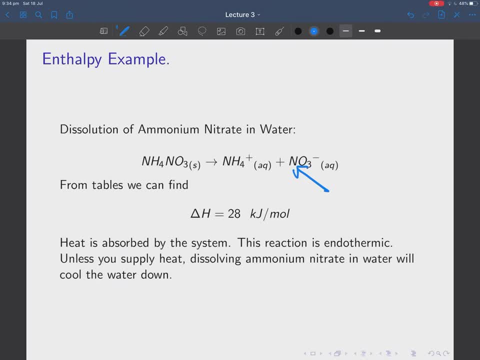 to our ammonium nitrate dissolution problem. Here it is And from the tables we find out for this reaction. I'm not going to show you how to use the tables because we're not doing a chemistry course- that delta H is 28 kilojoules per mole. 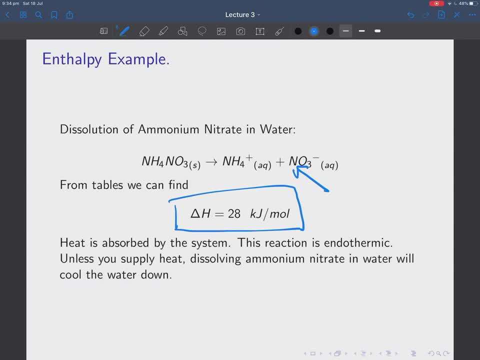 Okay, So delta H is 28 kilojoules per mole. That means this reaction requires amount of heat per mole of 28 kilojoules to go forward When it goes forward. that's how much heat it requires, Okay. 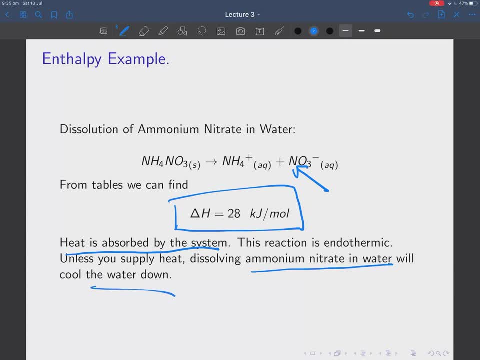 So this reaction is endothermic. Okay, And unless you supply heat, dissolving ammonium nitrate in water will cool the water down. So you throw the ammonium nitrate in and it will. it will cool down, Okay. 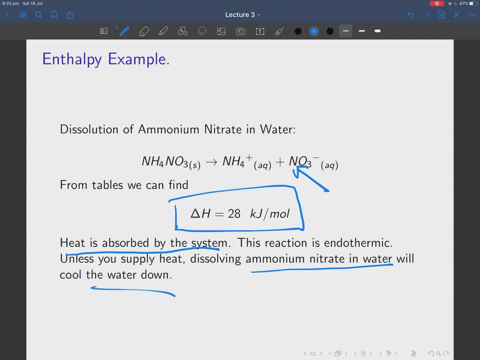 It's an endothermic reaction. Okay, So there are some reactions, you know in in in chemistry, Even the dissolution ones. you just mix, you know you put acid in water. it heats up, for example, That's. 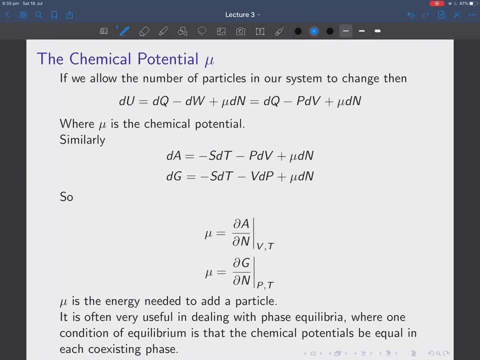 that's exothermic, It's endothermic, It absorbs heat. Okay, So our final um chemical, our final thermodynamic potential is the chemical potential mu, which we will have a lot more to do with when we do with. 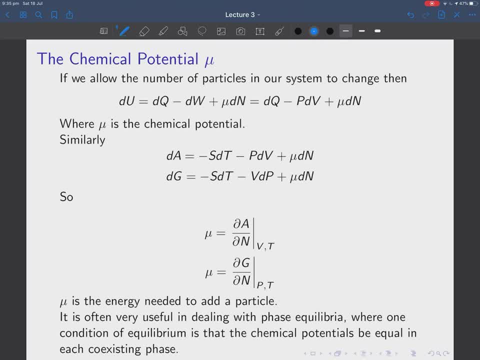 poles, bosons and fermions. Um but um. chemical potential mu arises from something we haven't really allowed for before, which is to allow the number of particles in our system to change. So the first law is now written. 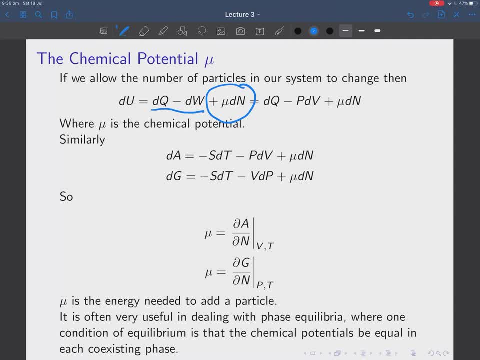 as dq minus dw plus mu, dn. Okay, And mu here is called the chemical potential. So this guy is the chemical potential, Okay, Invented by Gibbs himself. Okay, And similarly you can go rack and derive what? uh. 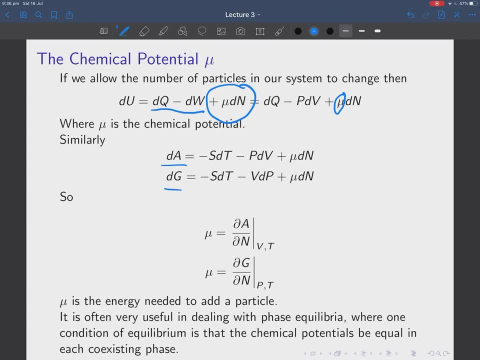 change in Helmholtz free energy or Gibbs free energy is Okay. Uh and mu here is um, dAdn at constant Vnt or dGdn at constant Pnt, um or uh, dUdn at constant. 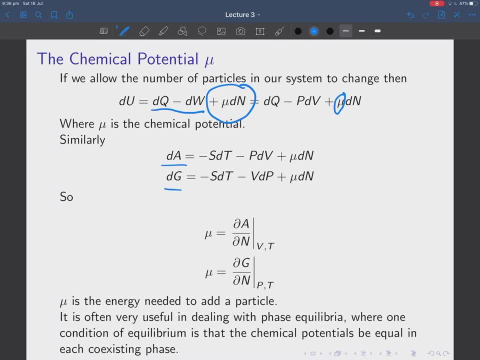 uh Vnq. Okay, So um, its usefulness is that it's the um energy involved in adding a particle Um and it's very useful in dealing with phase equilibria where you have different coexisting phases. 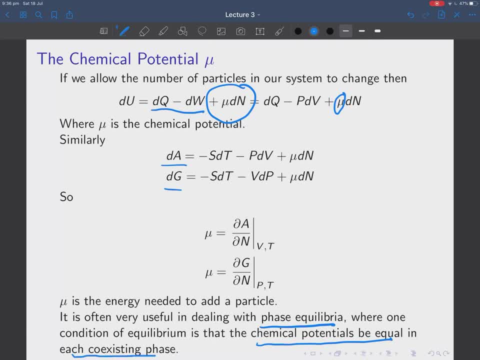 And one. one condition of equilibrium is that if you can exchange material, the chemical potentials must be equal in each coexisting phase. So I've got two phases. Suppose you've got phase one and phase two, and I have um some atoms. 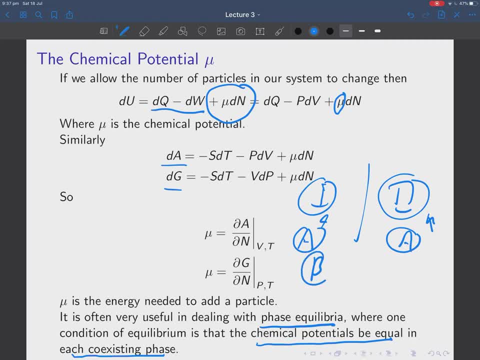 of of type A. The chemical potential of the atoms of type A here must be equal to the chemical potential of the atoms of type A here in this side, And similarly if another atom's of type B. it must be like that. 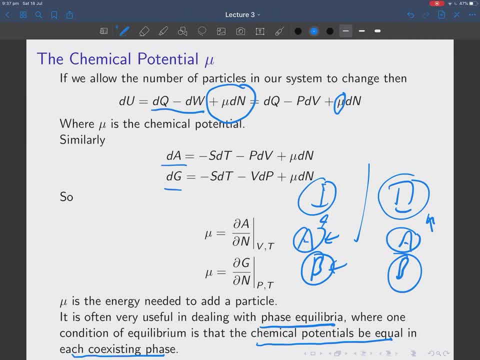 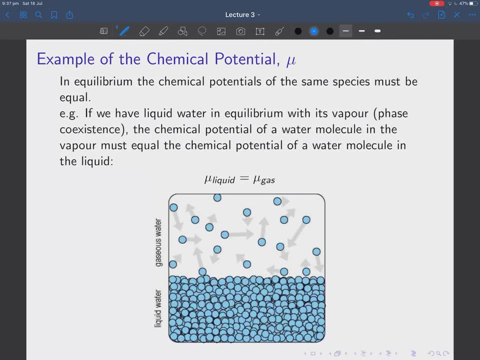 Okay, So this, this one could be nitrogen, A could be nitrogen, B could be oxygen. If you have two separate phases, one might be ice, one might be gas, and the chemical potentials be equal for each species across the boundary. 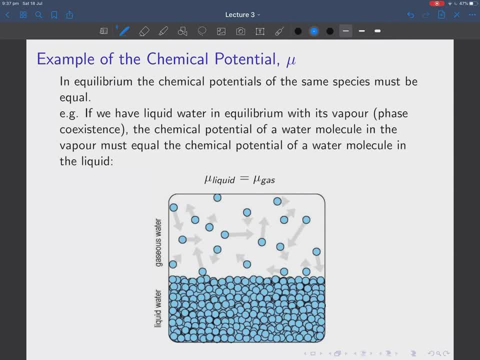 across the phase boundary. Okay, So one example. let's do a simple example of that Um. if we have um, as I said here, the chemi- in equilibrium, the chemical potentials of the same species must be equal. 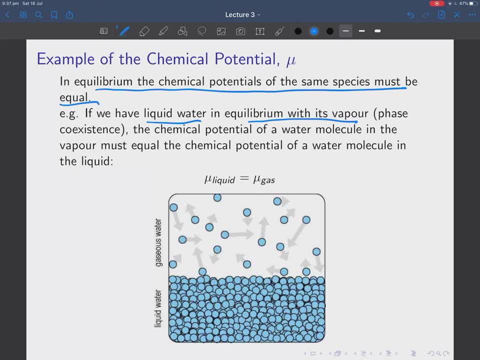 Okay. So let's take a case of liquid water in equilibrium with its vapor, which we will study quite soon. Okay, So you, you take a container, at certain temperatures, a liquid water, and it will have, suppose there's no. 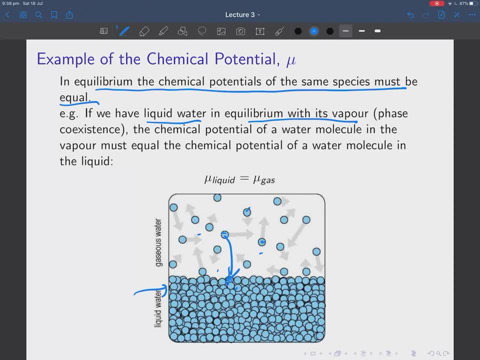 no air here, just water vapor, And that will. those two things will be in equilibrium, Some will constantly. you'll have uh the vapor colliding with the uh the liquid, uh and liquid bits coming out and forming the vapor. 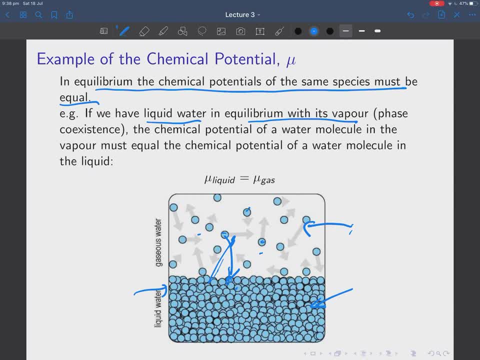 There'll be an equilibrium. There'll be some vapor and some liquid. Okay, What I just told you is the chemical potential of a water molecule must be the same here as it is here, Okay. So if you know the formulae for the chemical potential, 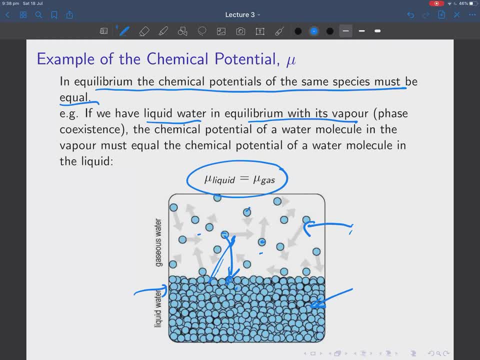 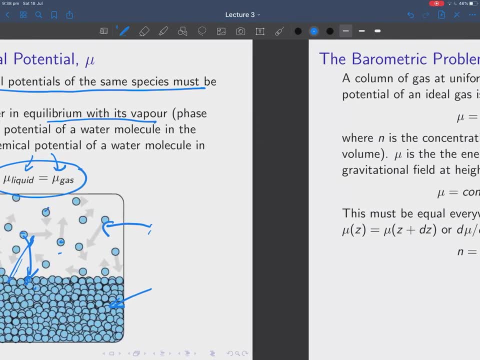 in each case. you can calculate, for instance, what must be the vapor pressure, et cetera. So mu liquid must equal mu gas. The chemical, the chemical potential is the input for each molecule must be the same in both cases. 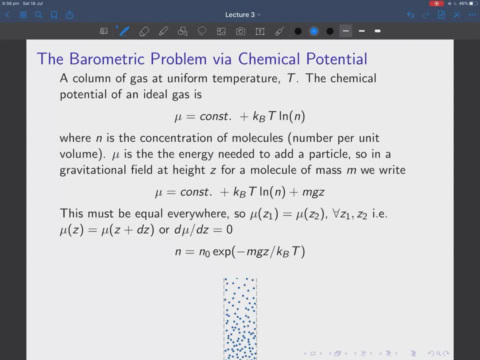 in both phases. Okay, That's. that's a very simple hand-waving um situation. Now let's look at um a more complicated calculation, which you've done before. okay, So you're familiar with the barometric problem. 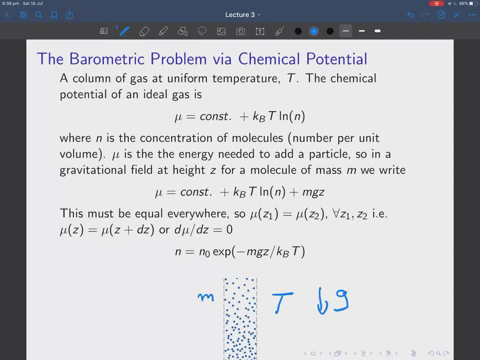 where you have an atmosphere which is isothermal and there's a gravitational field G pointing down uh, and you have some molecules of mass M and you want to figure out what the density of this system is as a function of height Z. Okay, 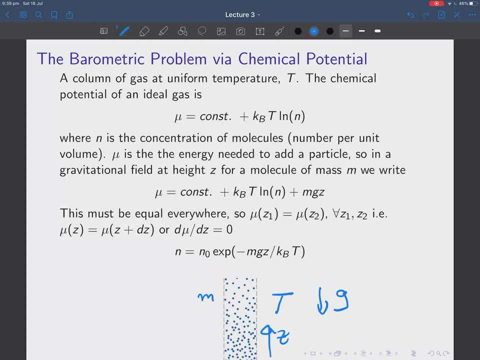 And I know I'm pretty sure most of you will have seen this problem before- We're going to attack it by using chemical potential. Um, now, later on, I'm going to show you how to do it. Okay, So what we're going to do. 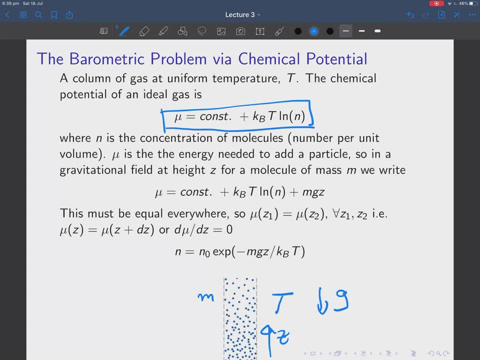 is we're going to use KBt times, the number of molecules per unit volume Now, which of course means it's still the KBt times- the log of the pressure, or log of the density, or whatever. Okay, But here we're going to use 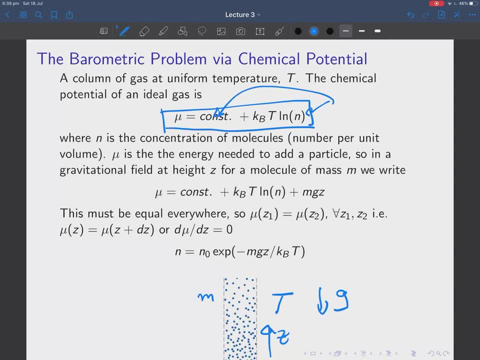 the number of molecules per unit volume. Okay, And you might say, oh, you can't take N and log N here, because you know things still is. is fine Now. um mu is the energy needed to add up one particle.